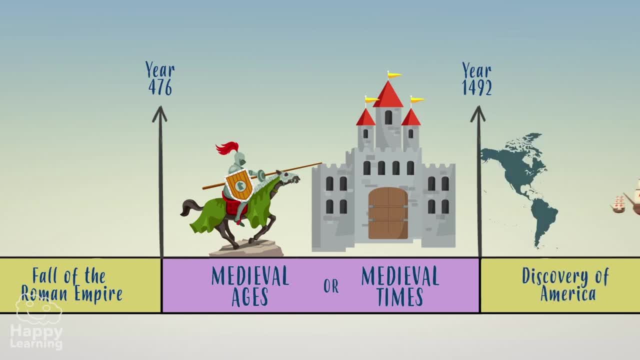 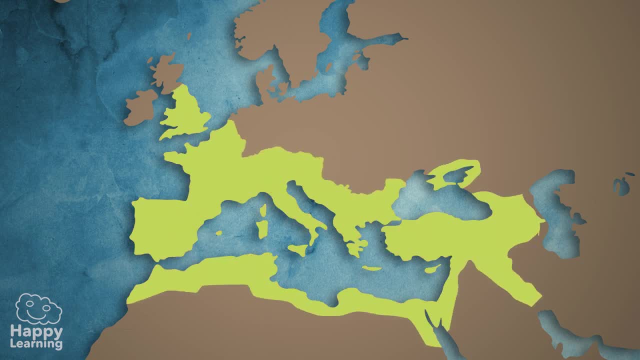 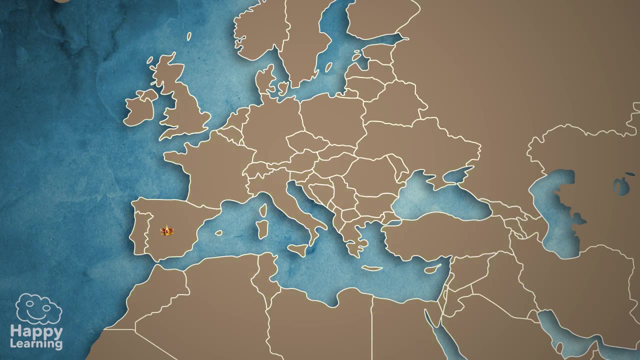 in 1492, with the discovery of America. In medieval times, the great territory dominated by the Roman Empire in Europe broke in many different ways and in many of them a monarchy was born, which is the form of government when a king or queen is in power. 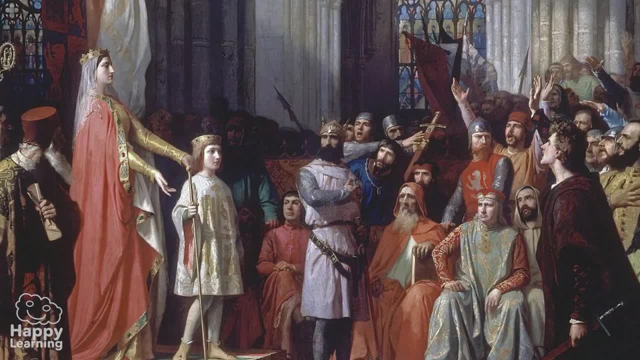 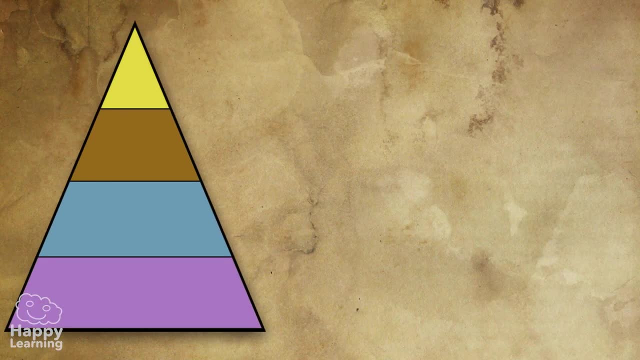 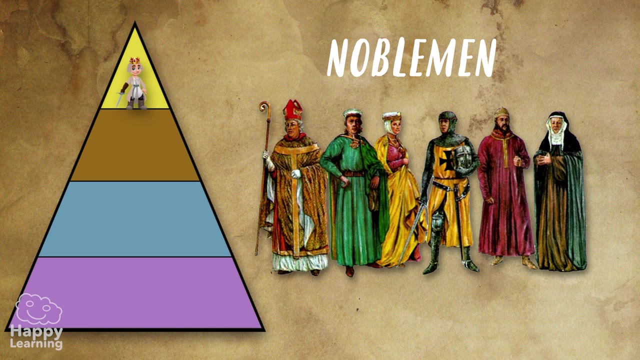 Royalty had absolute power and received their authority because of the feudal system. This system was based on a pyramidal structure. Royals were the most powerful of all. at the very top, Noblemen were just under, formed by counts, dukes, barons and other gentlemen and ladies. 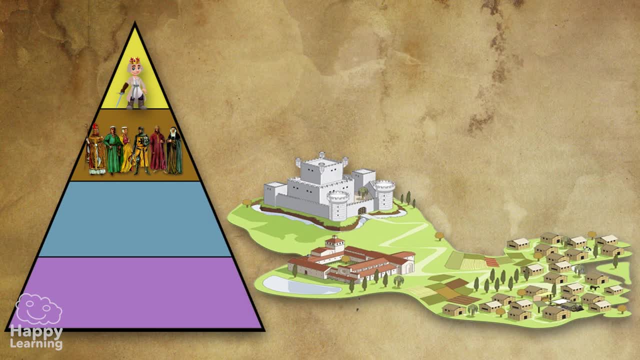 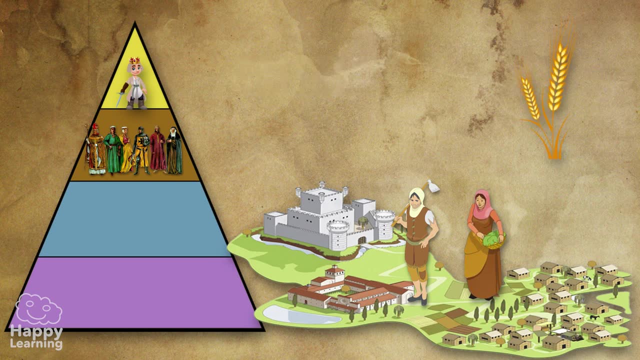 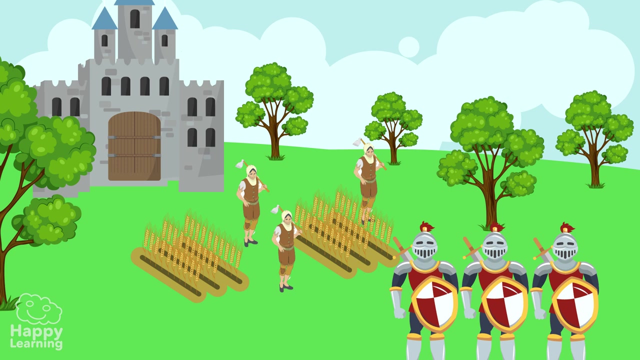 that controlled territories. Among the valiantist were the vassals, who worked and lived in the lands dominated by the noblemen and gave part of their work in exchange for protection and help. When they were attacked by enemies, vassals would run to the noble's castle. 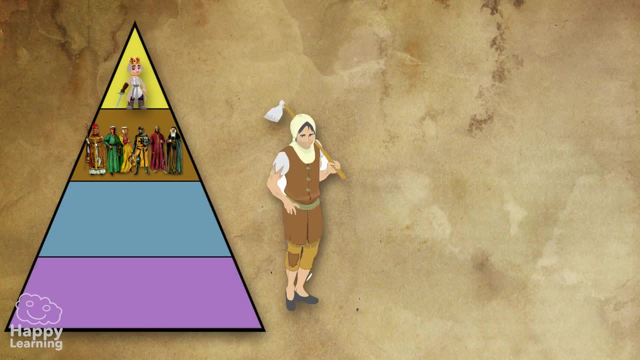 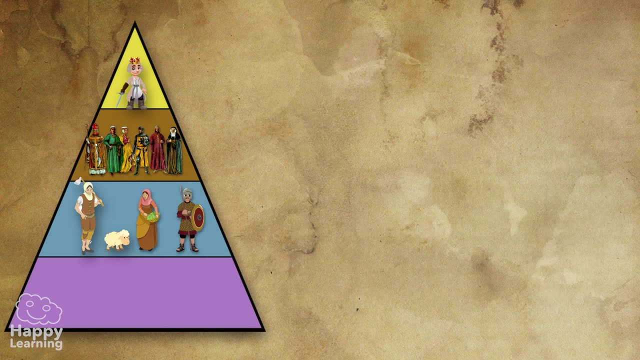 Vassals were farmers, shepherds, craftsmen and soldiers who were considered free men. The noble had the power to remind them of their own ghosts. Vassals would fight when they were attacked. The vassals would be responsible for protecting and saving their citizens. 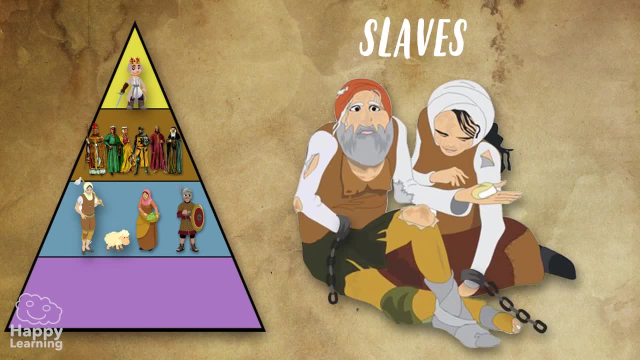 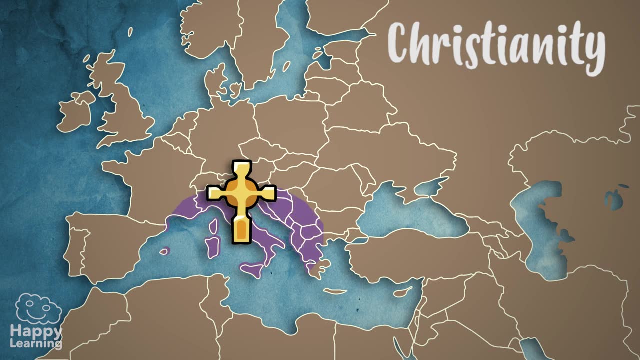 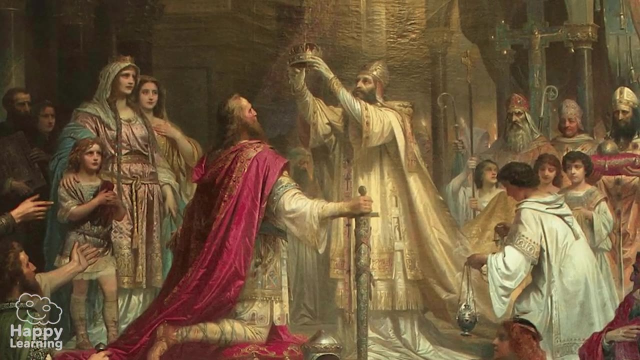 slaves were found, who were often war prisoners and would do the toughest jobs in exchange for nothing. Christianity was the religion that dominated Europe during the medieval ages, and its power was tremendous. Only the Pope in Rome was on top of the kings. The Pope acted like another. 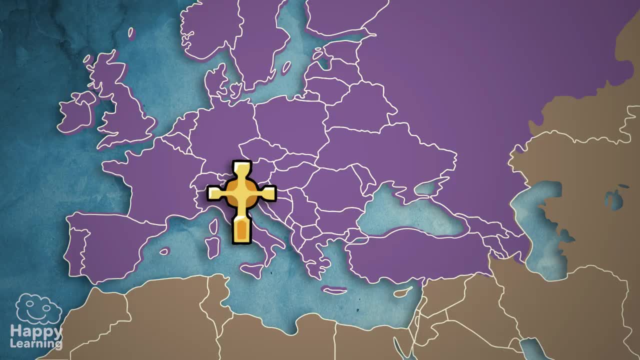 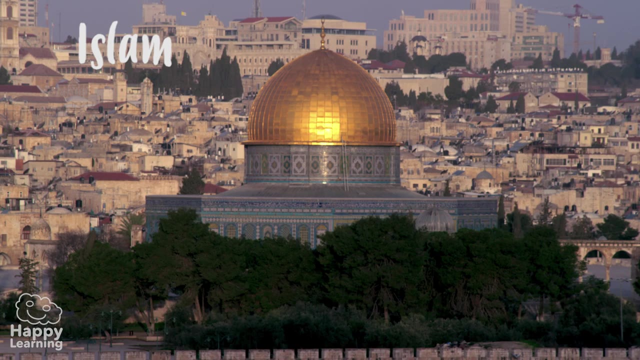 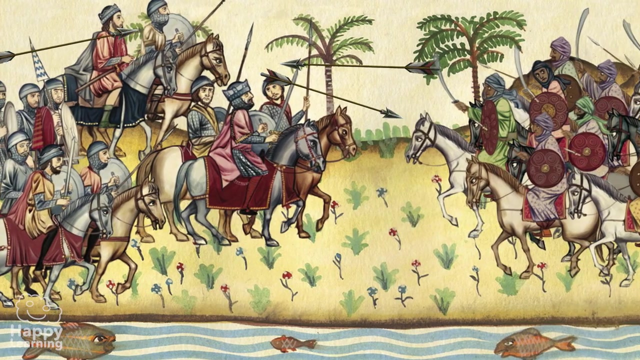 king. he controlled territories, formed alliances and declared war. The most important wars were the Crusades, where European knights and their troops tried to dominate the sacred land dominated by Muslims. Islam was another great religion during this time, and confrontation between Christians and Muslims was constant. 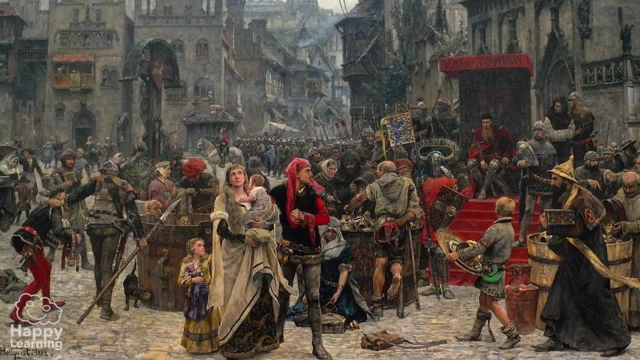